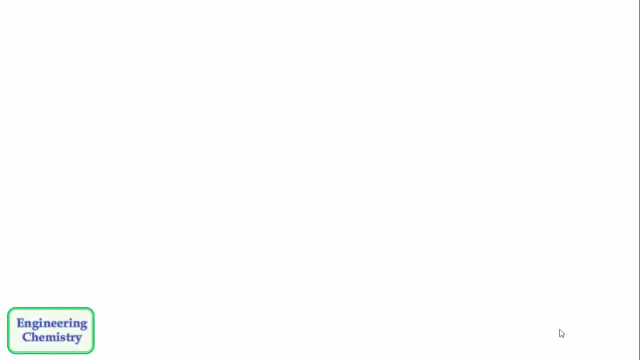 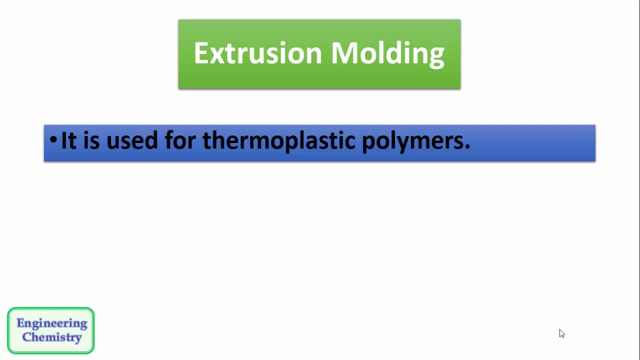 Hello friends, welcome to engineering chemistry. Today we are learning extrusion molding. Extrusion molding is used for the linear polymers. Most often it is used for the thermoplastic polymers. Using extrusion molding, long articles are manufactured. Let us understand the process. 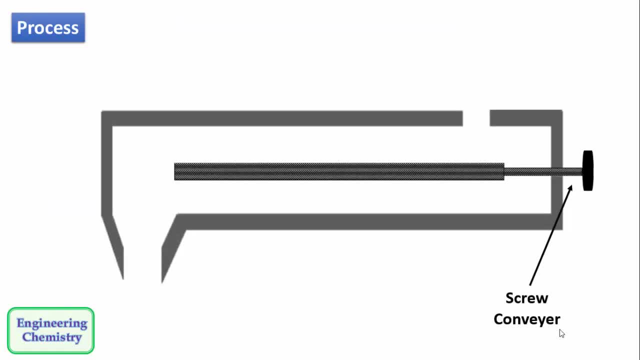 of extrusion molding. It consists of a machine with a screw conveyor. On top it has a hooper in which all the plastic ingredients are taken. Then it has the heater to melt the plastic ingredients. So first the plastic powder or granules of plastic is placed in the hooper. 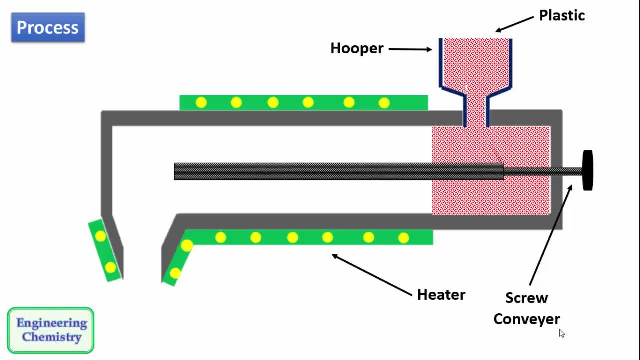 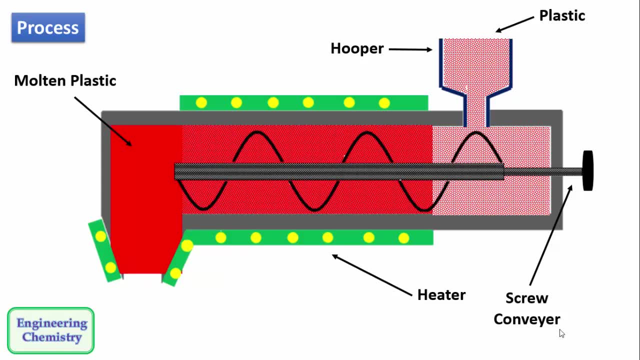 and then it falls into the machine. When the screw conveyor is rotated, the plastic ingredients are pushed into the heater region where it melts, and finally, at the end we have the molten plastic. And when the metallic wire is introduced at the end of the machine, 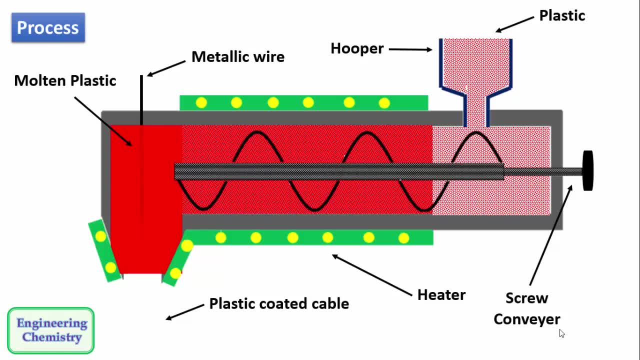 we get plastic, Plastic coated cable or electrical wire. that is how the softened plastic is forced through a hole in the extrusion die. The extruded plastic is cooled. that is the curing process is carried out, and that is how the long articles are produced and then cut into the desired length. 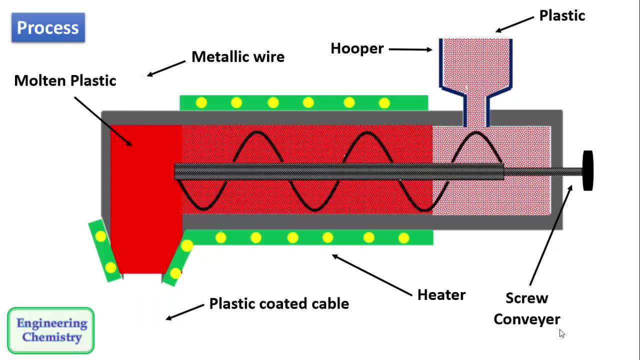 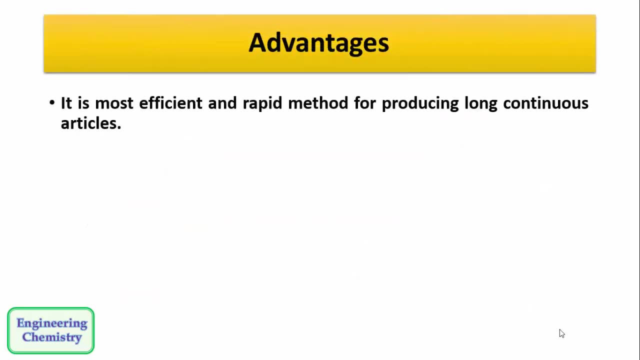 The shape and size of the extrusion is the same as the shape and size of the hole in the die. So by changing the shape of the hole in the extrusion, die will produce different shapes of particles. Let us see the advantages of extrusion molding. It is the most efficient and rapid method for producing long, continuous articles. 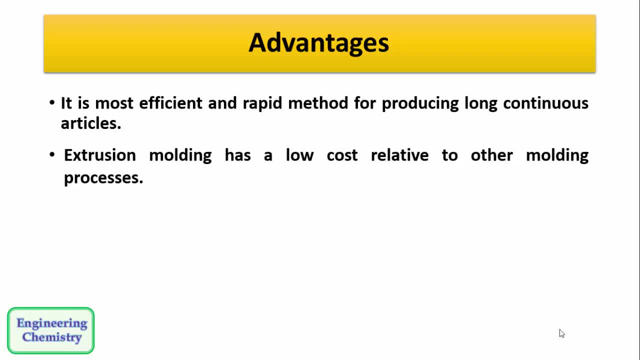 Extrusion molding has low cost relative to other molding processes. Extrusion molding provides considerable flexibility in manufacturing products. That is how the flexible electrical wires are produced And, the most important thing is, the plastic remains hot when it leaves the extruder, Which allows for post extrusion manipulation. 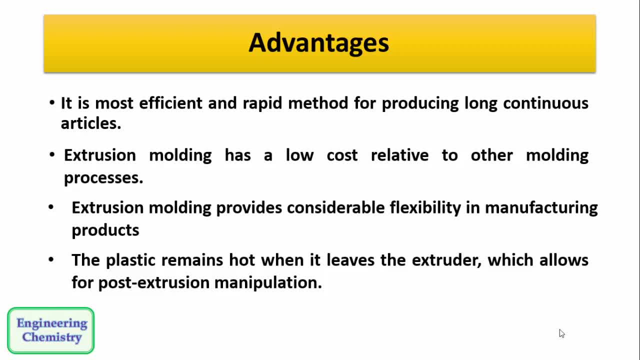 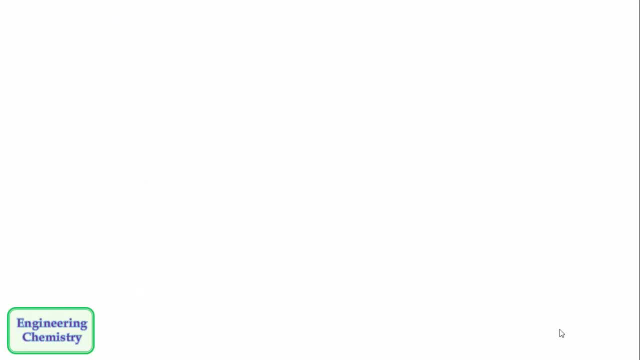 That means even if the plastic leaves the machine, it remains in the hot condition, So it allows us to change the shape of the article when it comes out of the machine. Let us see the disadvantages of extrusion molding. The first is it can be used only for linear polymers.